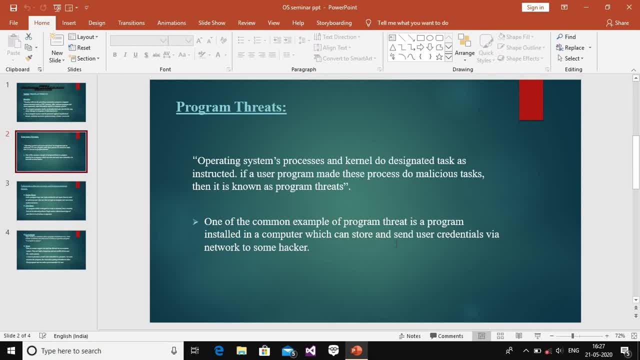 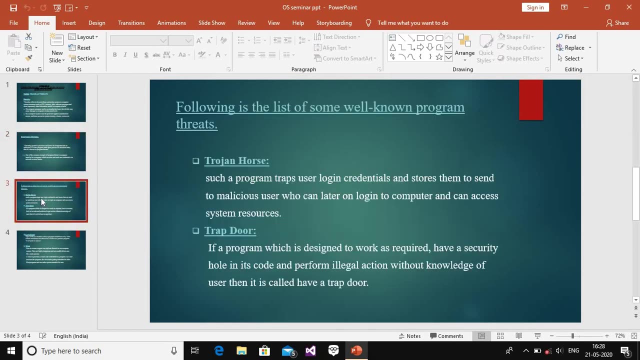 program thread. you know, we can installed in a one of the program on the computer. it should be store or it should be sent to the another credential network. okay, this, some hacker, this example for the program threads. okay, we are going to the next concept, then some of the well-known program threads. some of the well-known 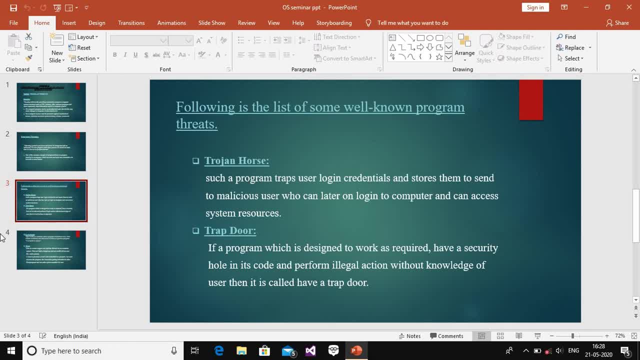 okay, usable program threads like the first one is Trojan arts. frozen arts means such a program traps user login credential and store them, send to the malicious user who can later on log into the computer and can the system resources. the firstly the one of the user can program traps on the. 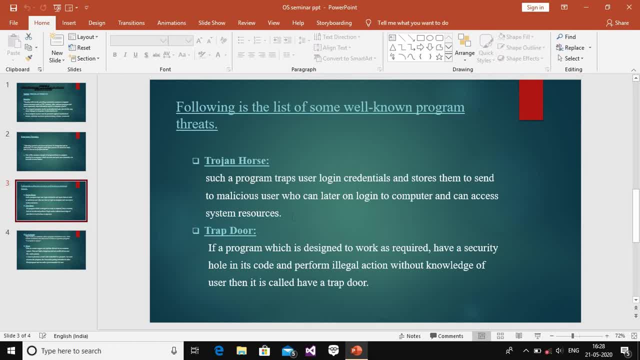 credential store. okay, it should be malicious user. it can be stored in the computer and after some times, later, another user can log into the system and to access the resources. okay, this means the trojan horse. okay, the next. next one is the trapdoors. the trapdoors means if a program which designed to work as 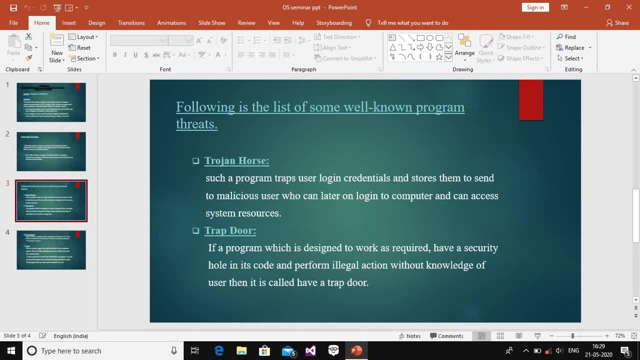 required security holds code and perform illegal actions without knowledge of user, then called a trapdoors. this means the summer code and perform code and perform illegal actions. some misbehaves, some another without knowledge user can use this program. some security problems are arised in the system. this is called trapdoors. some problems are: 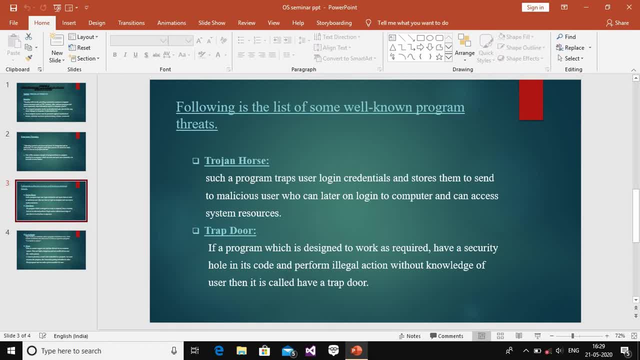 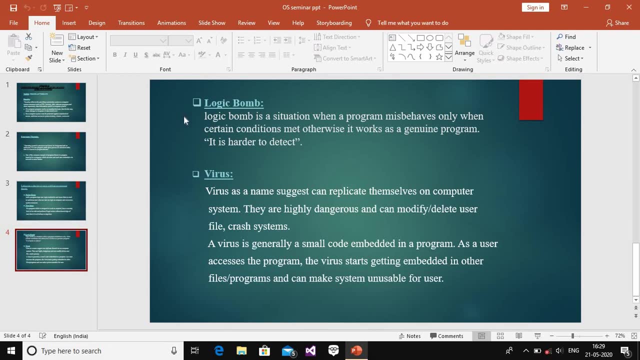 arised in their illegal actions, some without knowledge. persons are used in a program. this problems are arised in a system. this means called trapdoors. okay, we are going to the another program. threats, then logic bomb, the. what do you mean by logic bomb? the logic bomb means the it is occurred, the program misbehaves. 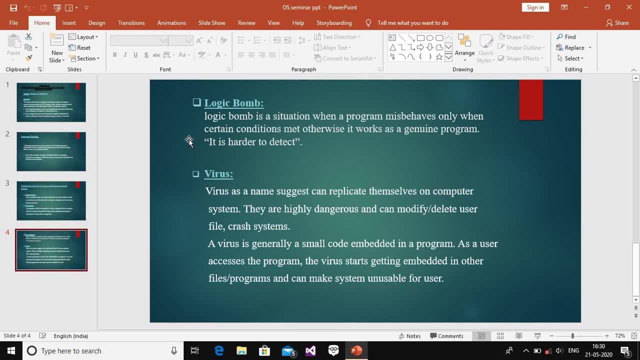 only a certain conditions, that other it. but it work, ruin and program okay. the logic bomb means it misbehaves only certain conditions, some conditions, only the problems are raised in the system. the anytime it will not occur. their problem, it is only some certain conditions. are the problem occurred in this program?